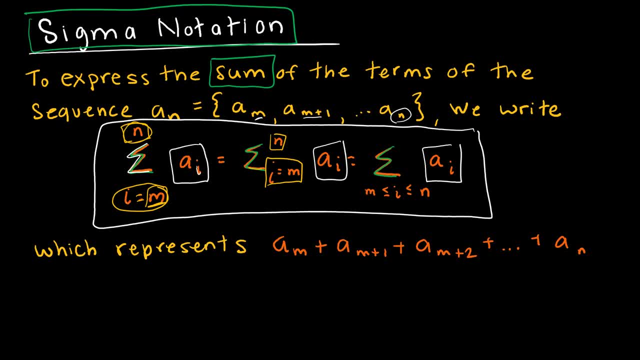 m. that's the lower limit up to n. But instead of above and below it's sort of to the right of, And the last way is written all below. So m is less than or equal to. i is less than or equal to n. All of those say we're going to start at m and we're 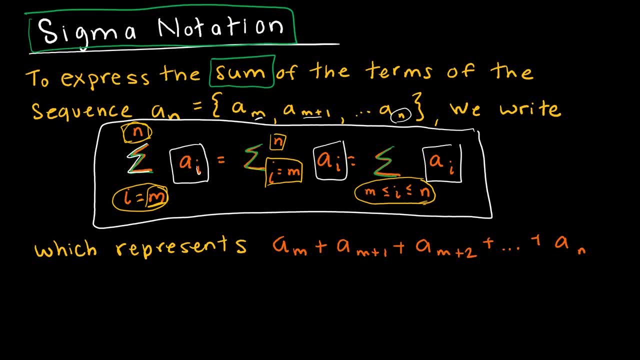 going to continue to increase by 1 all the way up until we get to n. So, again, any of these things say the same thing, and that says we're going to take a sub i, where i starts at m and then continues to increase by 1, m plus 1, m plus 2, all the way up until we get to whatever our upper value is. 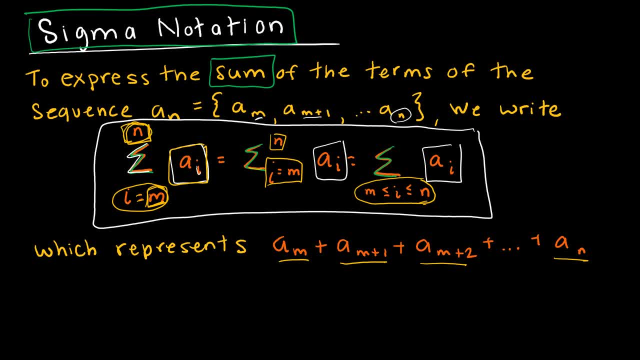 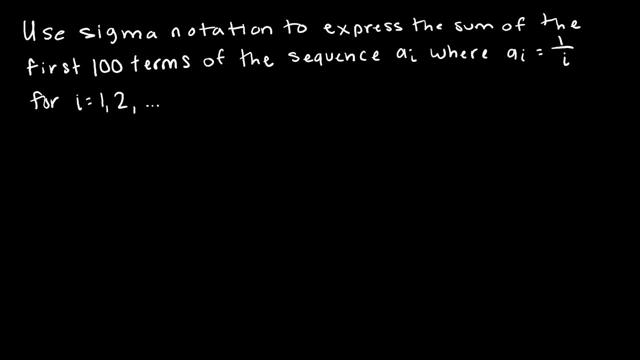 our upper limit. That's going to be the last one. Now, keep in mind we're looking for a sum. So this is saying I'm going to add all of these together and then in the end, I'll have some value. that is the sum. So let's do a quick practice for how to write something using sigma notation. 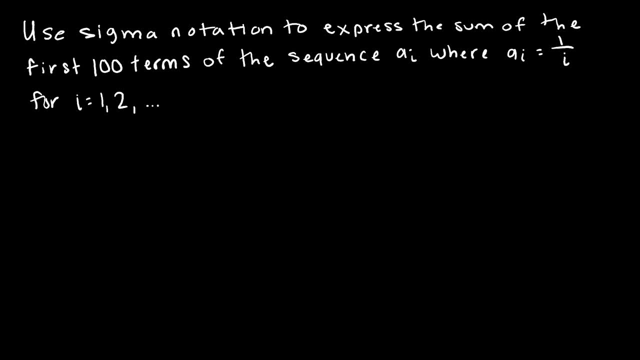 I want to use sigma notation to express the sum of the first 100 terms of the sequence: a sub i, where a sub i is found by taking 1 divided by i, For obviously starting with i at 1,, 2,, 3, etc. So before we use sigma notation, let's just take a. 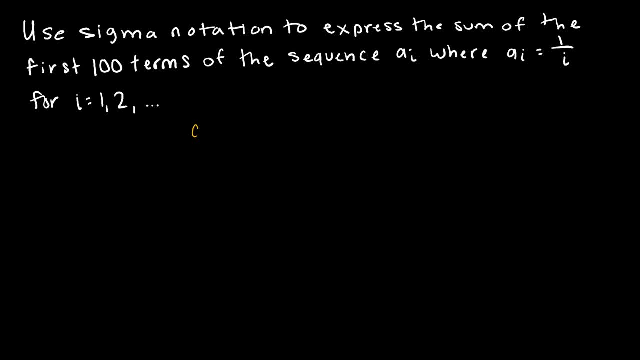 look at what this sequence looks like. a sub 1 would be 1 over 1.. a sub 2 would be 1 over 2.. a sub 3 would be 1 over 3.. So this sequence- if I were just writing the sequence, is 1 over 1,. 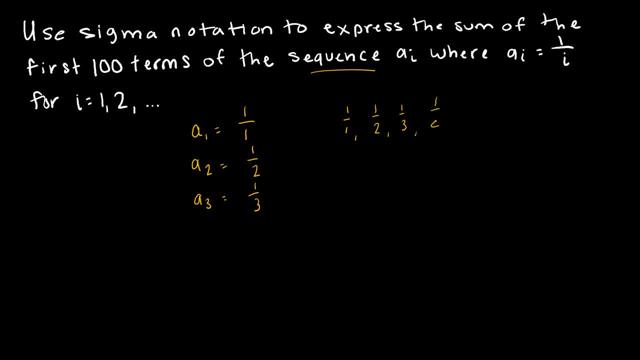 1 over 2, 1 over 3.. 1 over 4, all the way up to 1 over 100.. Now we're trying to find the sum of those first terms, So that would just be 1 over 1, plus 1 over 2, plus 1 over 3, plus 1 over 4, all the way up to. 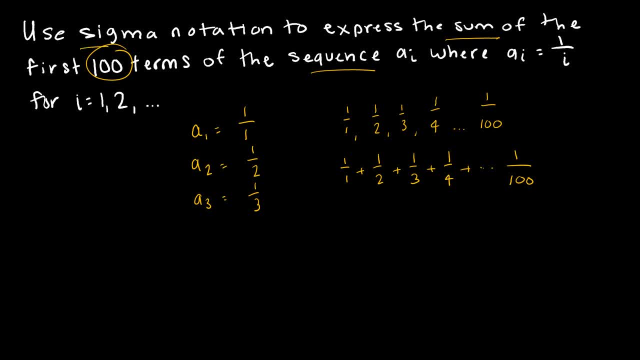 1 over 100.. But I want to do that in sigma notation, So I want to take this and instead write it as sigma notation. Of course we would use sigma And then below we would say: i is equal to 1, because that's the. 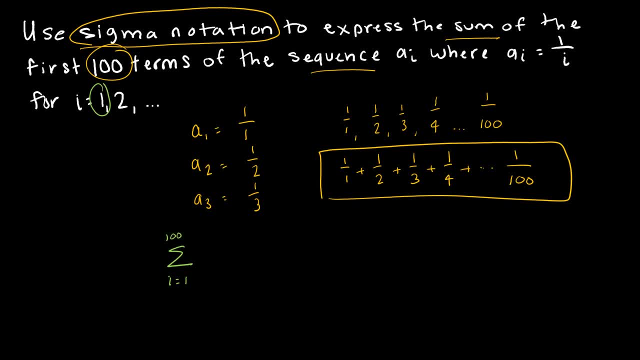 starting point and goes all the way up to our upper limit of 100.. So we're starting at 1 and going to 100.. And how are we defining those terms? 1 over i? So the important thing here is that the i here matches the i here, because that's what the i here is telling me to do is. 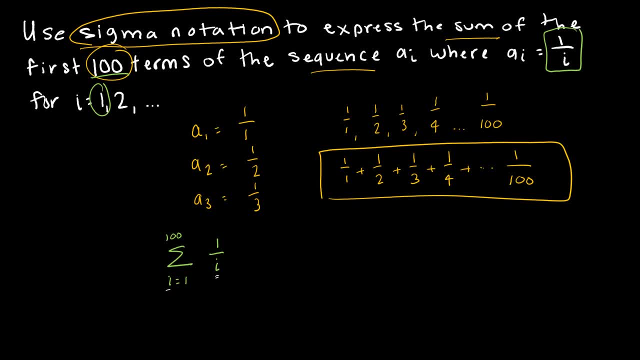 start at 1 and then continue to 100. So did I do this correctly? Well, let's take a look. This says start at 1 over 1 and then continue to increase that value all the way until you get to 100. So do these two things match? 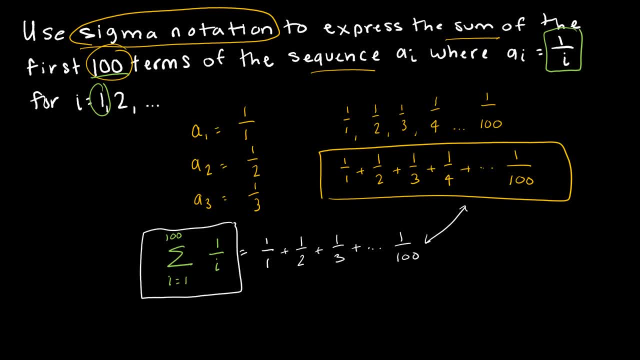 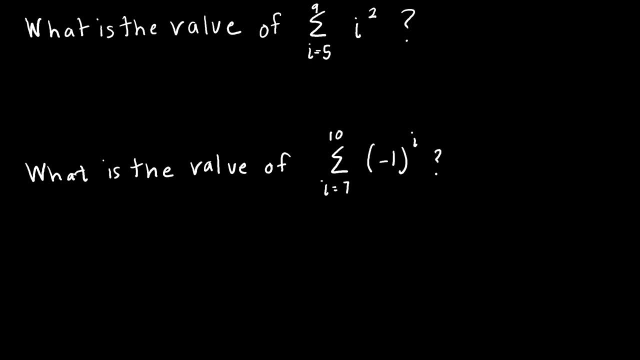 Yes, they do. So this is the proper solution for sigma notation. Two more fairly straightforward questions for us to go through together, just to make sure we're clear on what sigma notation is all about. So the first one says: what is the value of? 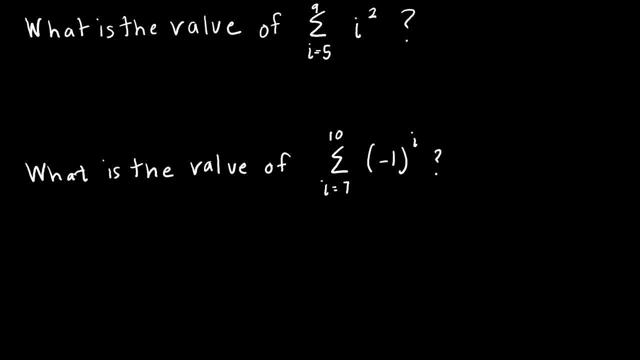 the summation from 5 to 9 of i squared. So all I'm going to do to find this summation from 5 to 9 of i squared is start at 5, increase that value and then continue to increase that value. 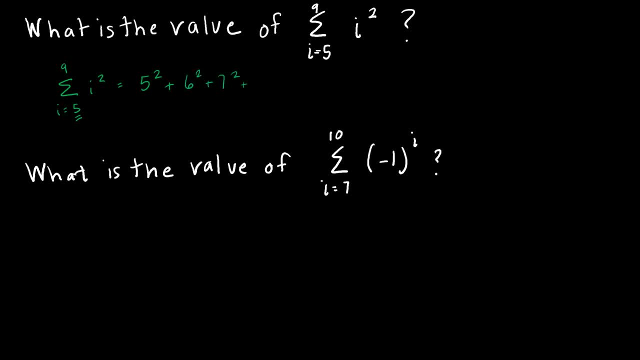 So all I'm going to do to find this summation from 5 to 9 of i squared is start at 5,, increase by 1,, increase by 1,, increase by 1, and stop when I get to 9.. 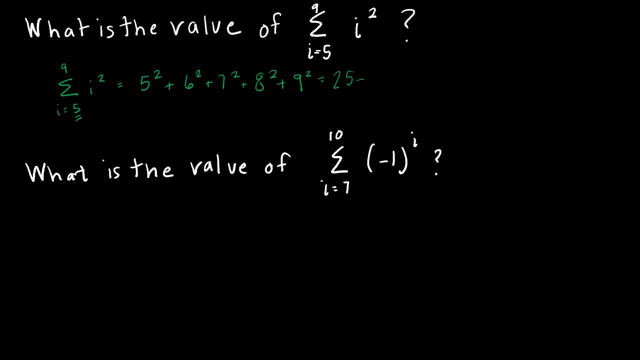 So of course that would be 25 plus 36 plus 49, plus 64 plus 81. And then I'm going to add those together to get to 55. So when we're asked to find the value, all we're doing is finding the sum by hand, essentially. 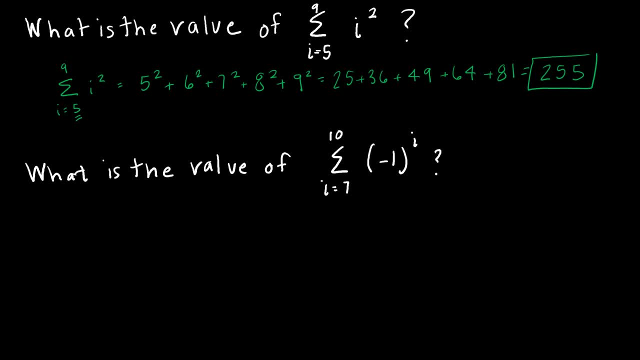 Same thing for the second question. This says the summation, as i goes from 7 to 10, of negative 1 to the i. So now i is the exponent, So I have negative 1 to the 7th because that's my starting point. 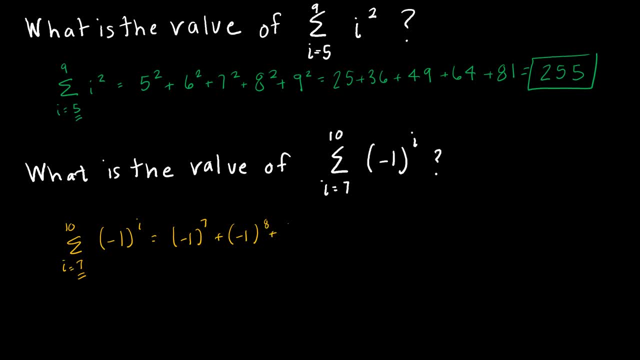 And then I'm increasing by 1, negative 1 to the 8th, increasing by 1, negative 1 to the 9th, increasing by 1, negative 1 to the 10th, And I stop at 10,.